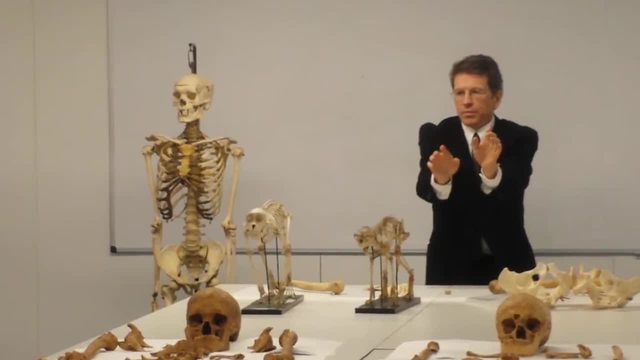 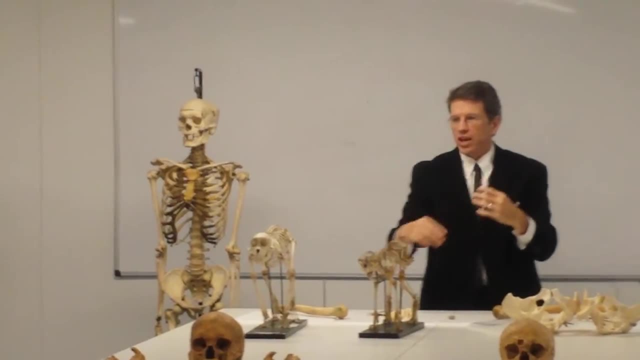 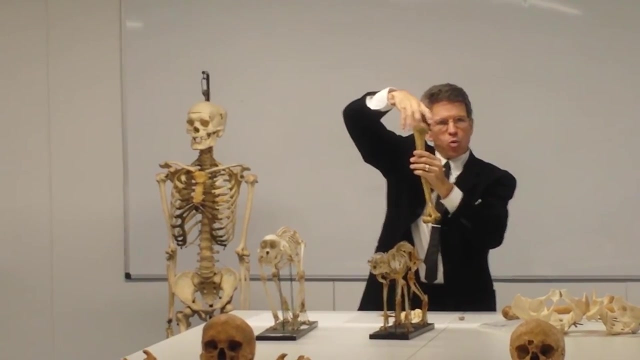 Apes can't do that. If you had that body, you couldn't get your arms above your head to grab hold of the branch Because your arm would be the wrong shape. So what happens in apes is the top of the humerus. this bit here has to turn, A quarter turn. 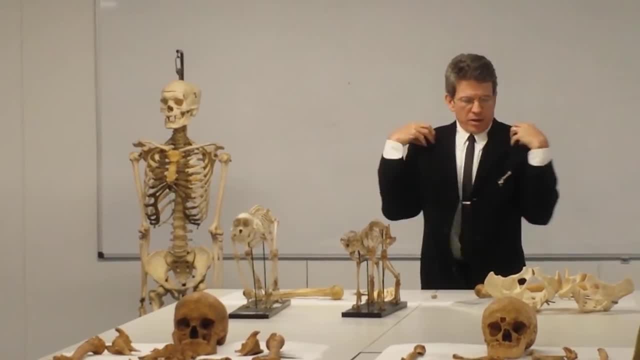 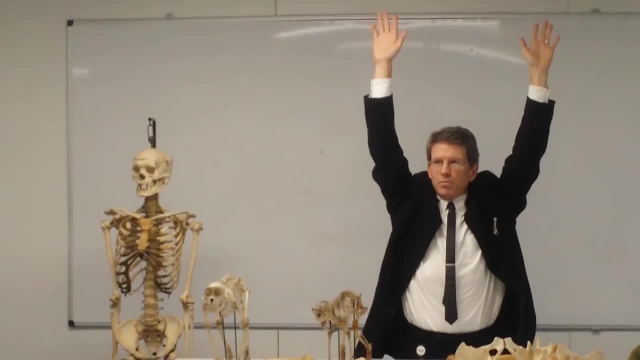 And over evolution. that's happened. That brings the shoulders from here to here, and it allows you to do an amazing thing: Raise your arm above your head. That's why baboons don't go to rays. You've never seen a baboon at a ray, have you? 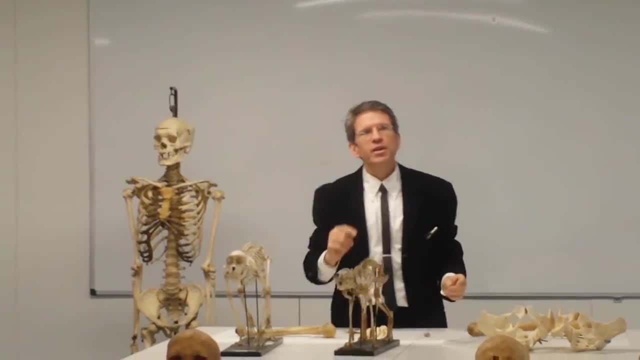 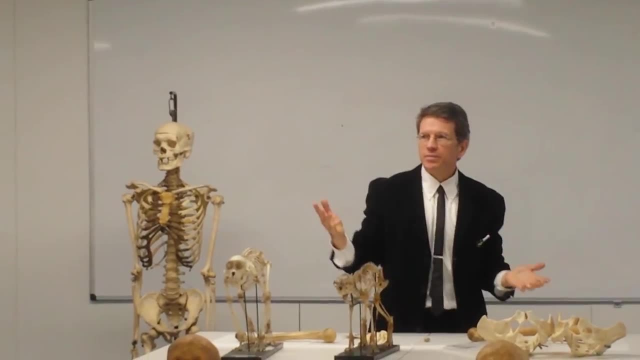 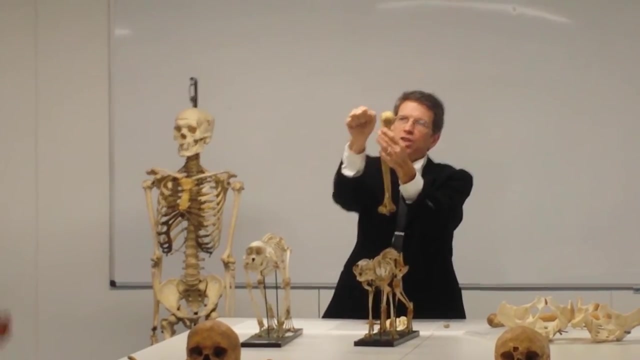 Right, Do you know why? Because when the DJ says, throw your arms in the air like you just don't care, he can't, He goes and he has to walk home because he looks stupid. So we can tell just from this part of this bone if it's got that quarter, turn in it to move the shoulder out to the side to allow them to go up and down. 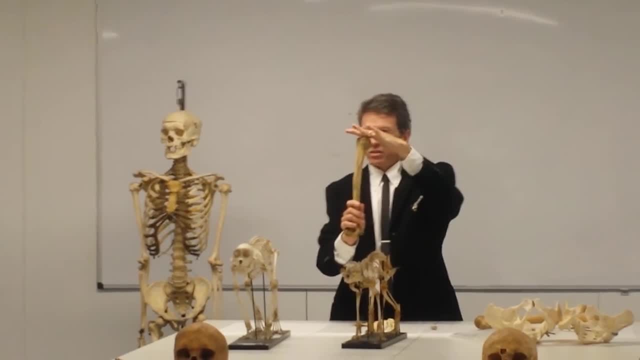 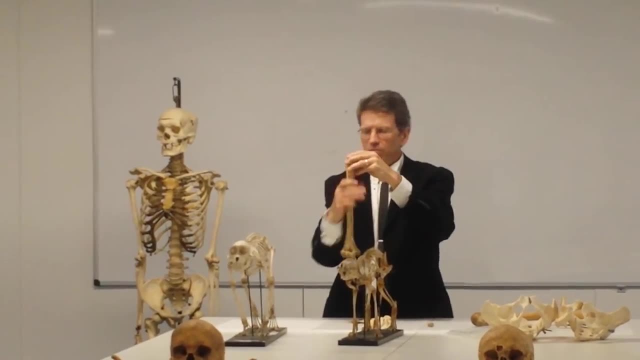 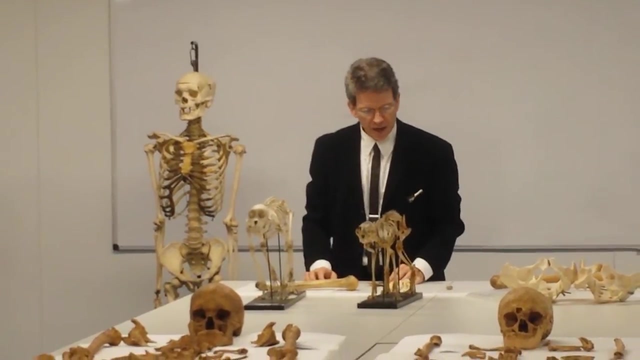 And we can tell that that animal is an ape And that change happened about 13 million years ago, Which is a reasonable number At that time, more than four or five, And that is something we can use to look at animals that are related to the group that we belong to, the apes. 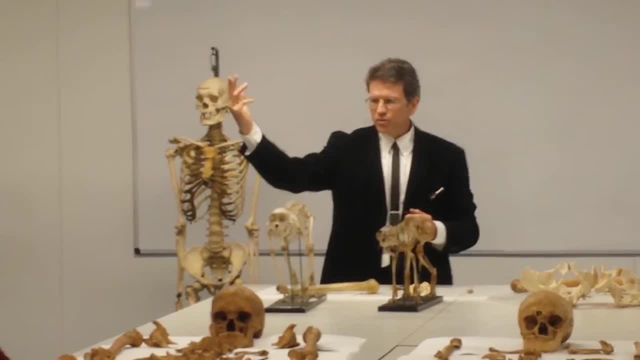 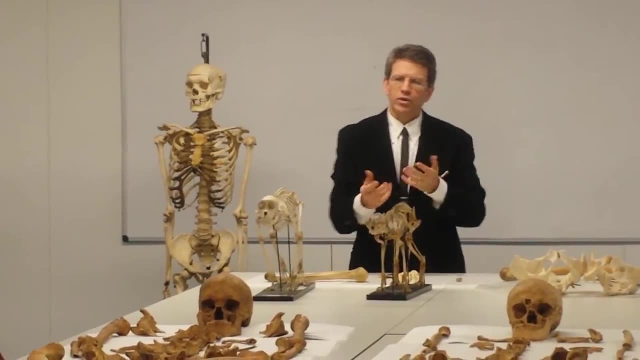 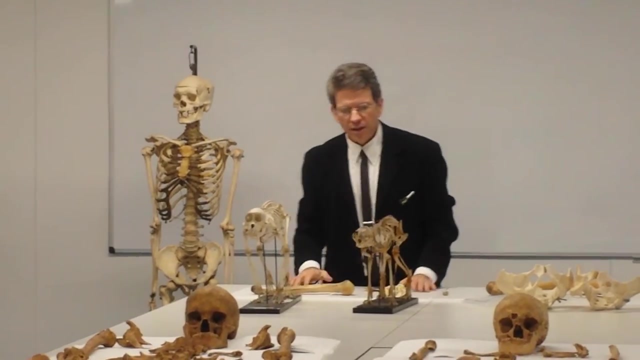 We also belong to a larger group which includes ourselves, the other apes and the monkeys, like this monkey here, and the lemurs and lorises, And that whole group is called the order of primates- primates, And we can also see some characteristics that we have, that we share. 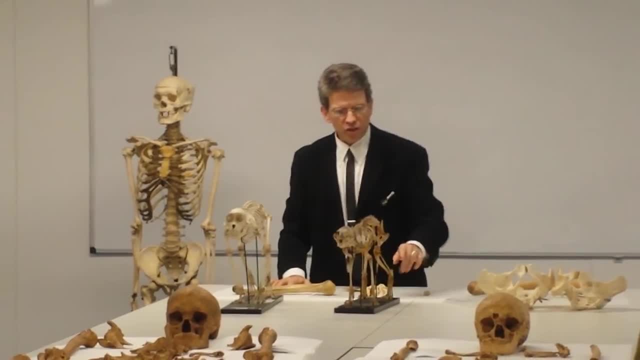 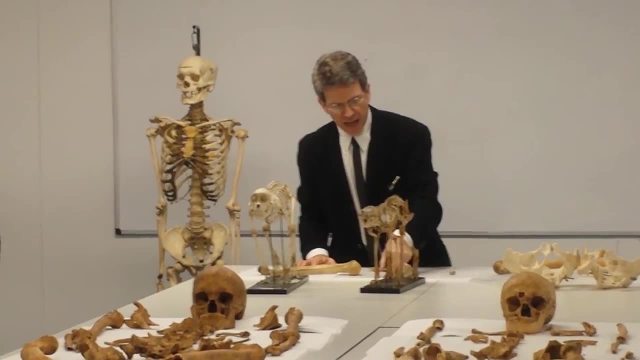 With the other primates which other animals don't have. So this animal here is a cat, And we shall call him Felix today, And cats are different from monkeys and apes and other primates in lots and lots of different ways. 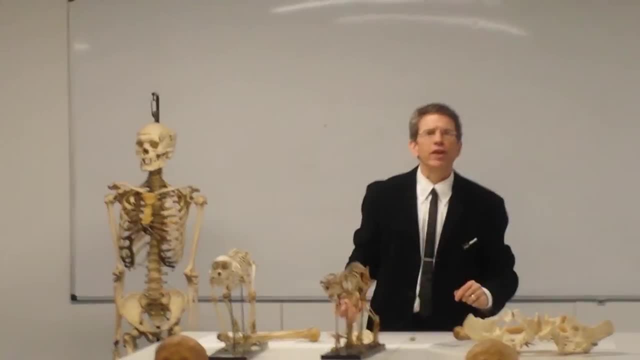 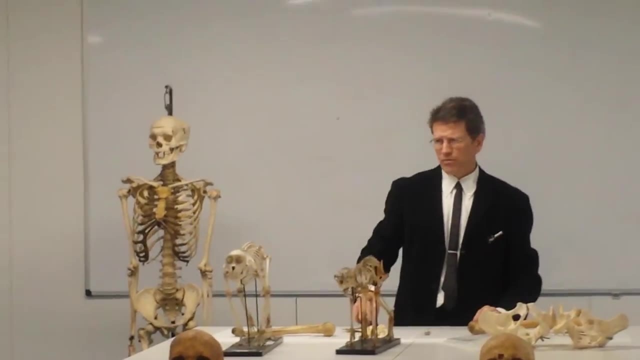 But one of my favorite ways has to do with their hands and feet. Okay, who's got a cat or a dog? What do you have, cat or dog? What's your cat's name? Kiki, Kiki, Female, I'm assuming. 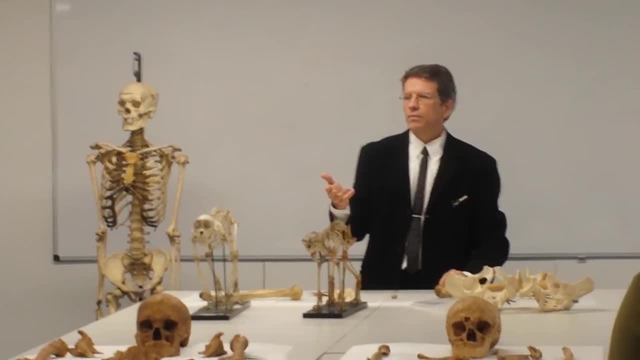 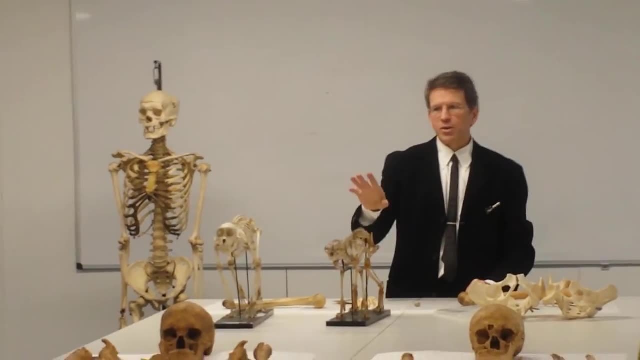 Yeah, What type of cat? A woman, I think it's a funny cat, maybe. Yeah, Ginger coloration. No, You have a pig's animal. It's brown, Brown. Okay, a brown cat, All right, Kiki. 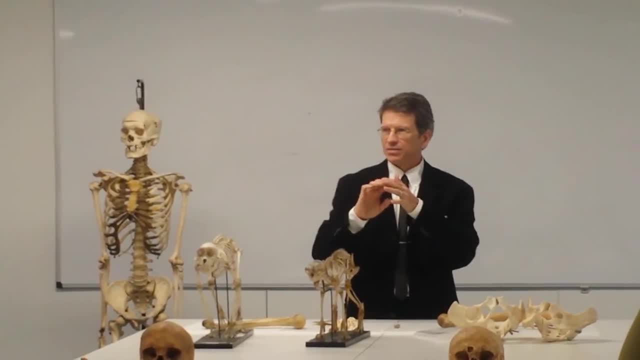 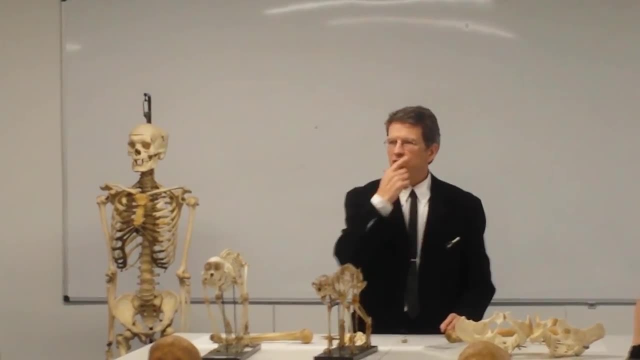 What's at the end of Kiki's hands and feet? Wait, Tail's on a hole in her part of the body. What? What's on the end of the hands and feet? Her nails. She doesn't have nails, She has claws. 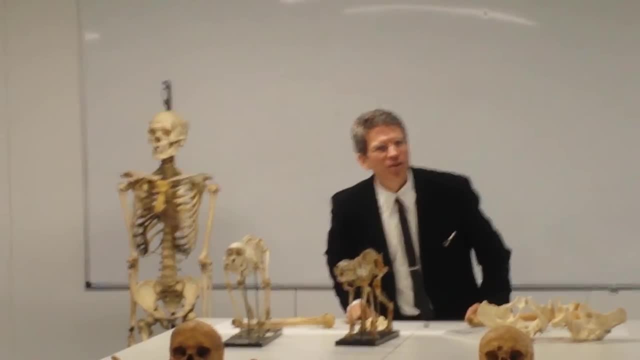 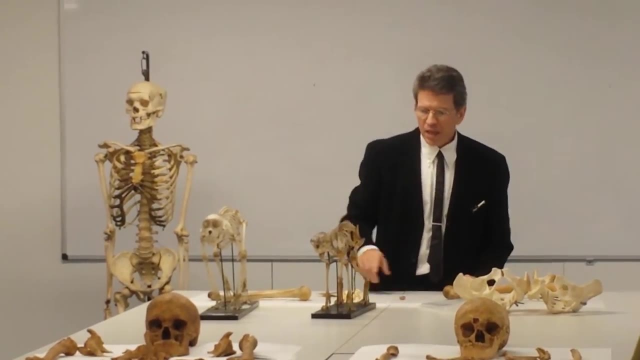 Claws, Claws, Claws, Claws, Claws, Claws And claws of a cat or a dog. That's what most animals have- Claws or hooves- And the bit that you see as the claw is the same bit that you have on your hands and feet. 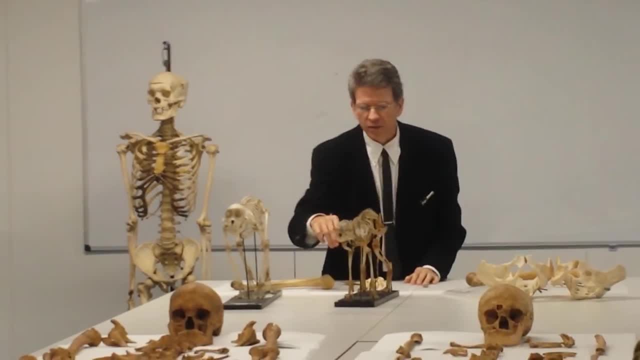 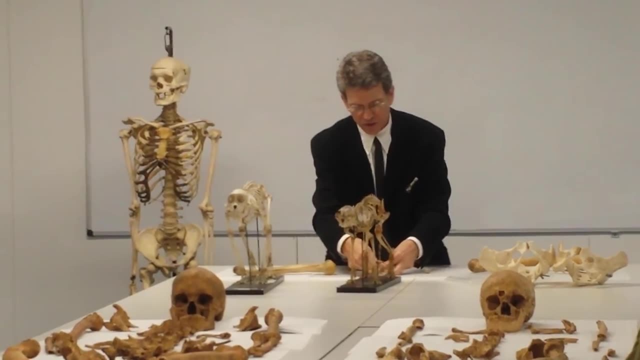 here, which is the nail, except it had a deep layer. that's slightly different and it's differently shaped. But what's significant about this in terms of looking at it in terms of fossils, which is what I'm interested in- is the bone underneath that. 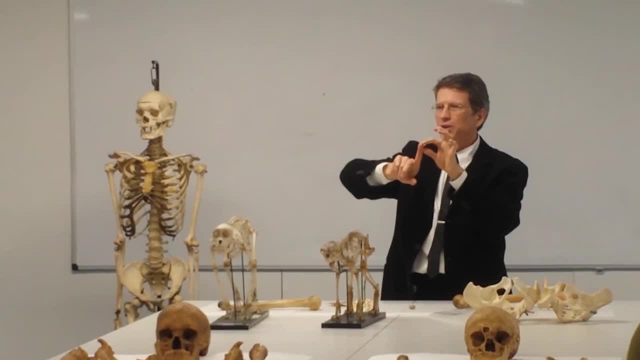 It's called a bone, It's called a phalanx. Ooh, Anybody know what a phalanx is named for? Anybody study Roman history? No, Nope, It's a group of soldiers. It's a group of soldiers like a wedge. 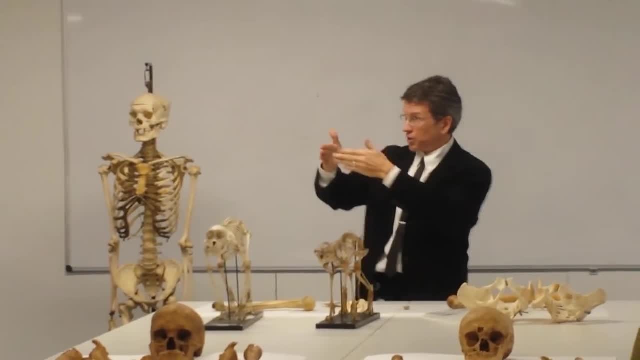 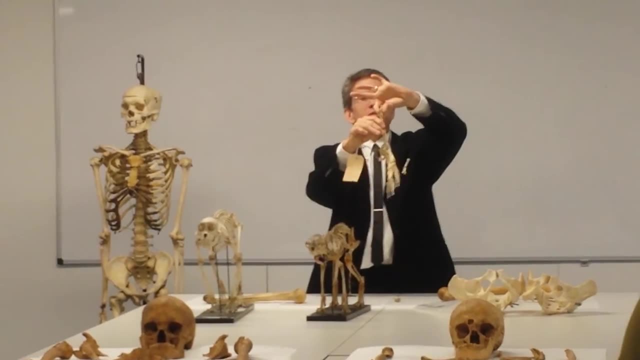 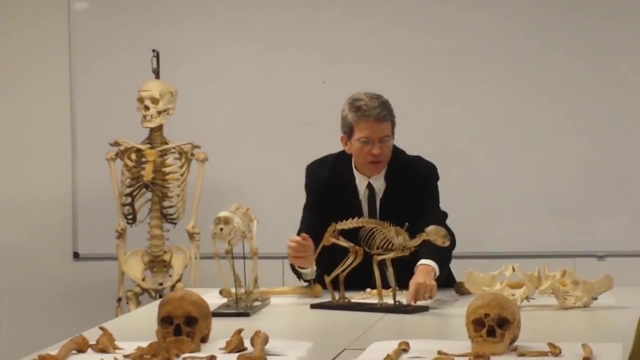 It turns out the phalanges, which is the plural, or phalanx, are little wedge-shaped bones at the end of your hands and feet, And in a cat or a dog those bones underneath the claw are claw-shaped. You can see here: 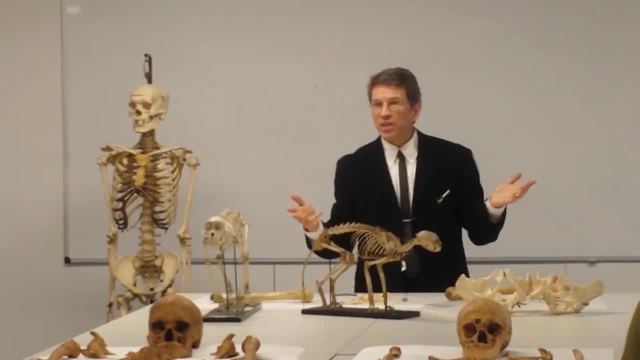 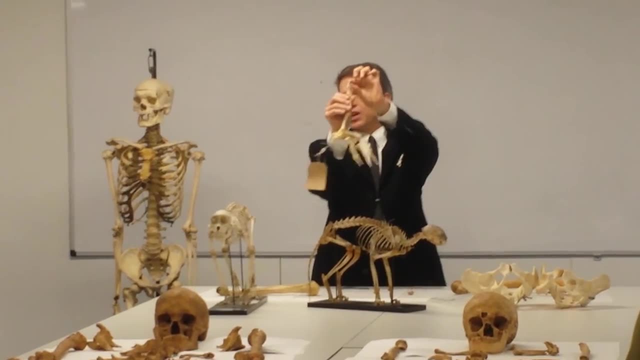 They're pointed and curved, And that's what most animals have. Primates, on the other hand, don't have that. A primate phalanx looks like this: It's a little wedge-shaped bone, It's flat and not looking like a claw. 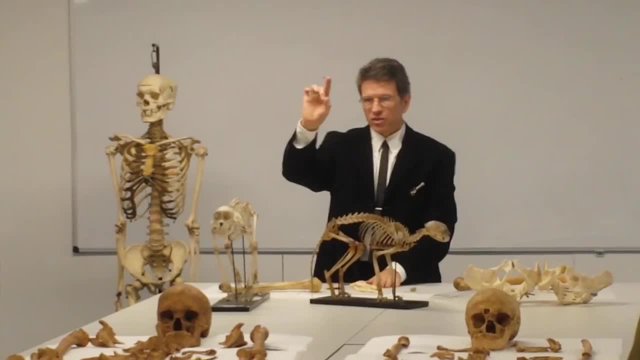 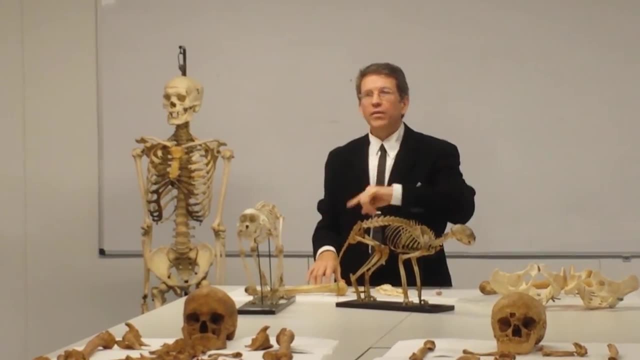 Why would that be? Why do primates not have claws and they have nails instead and flat fingers like that? Probably because they don't need them anymore, because they need to grip. They need to grip. Good point: You can do something amazing with your hand. 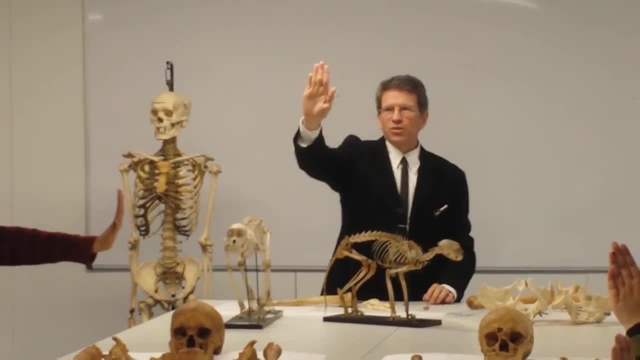 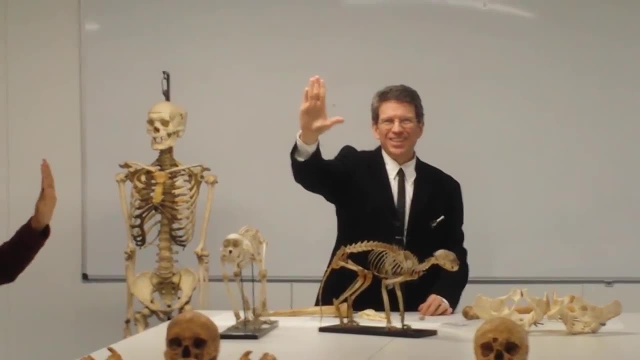 Put your hand up like this, You're going to do something that your cat or dog or horse or camel or any other mammal can't do. You can do this. Watch, Do that. Move your thumb away. Your bones have to be shaped differently in order to do that.